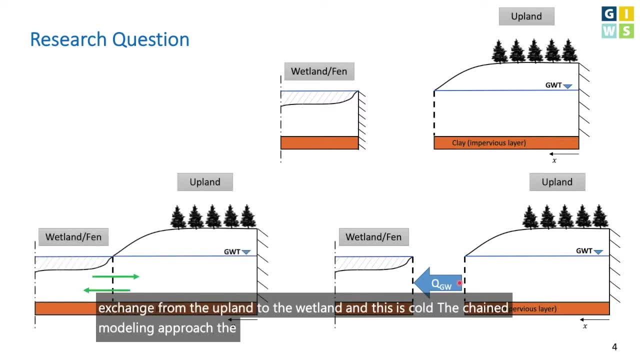 approach. The third approach is the full coupling between the upland and the wetland, which allows for a two-way interaction between both upland and wetland, And that approach would be the most accurate option, but also the most complicated. So the main question that we aim to answer in this study, 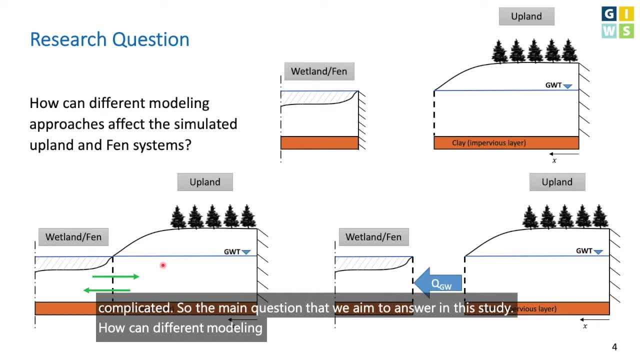 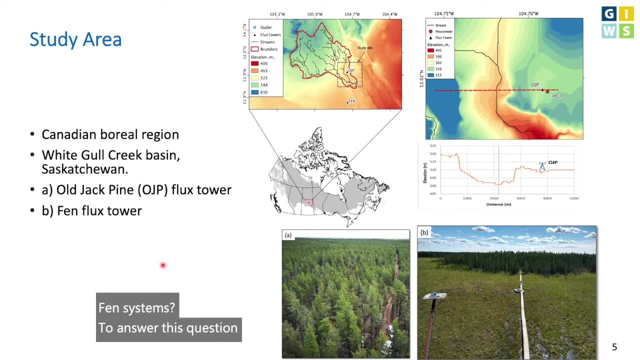 how can different modeling approaches affect the simulated upland and fen systems? To answer this question, we chose the study area in the Canadian Perrier region at the White Gull Creek Basin area in Saskatchewan, and mainly used the data from two flux towers. One is the Old Jack Pine, which represents the upland area. 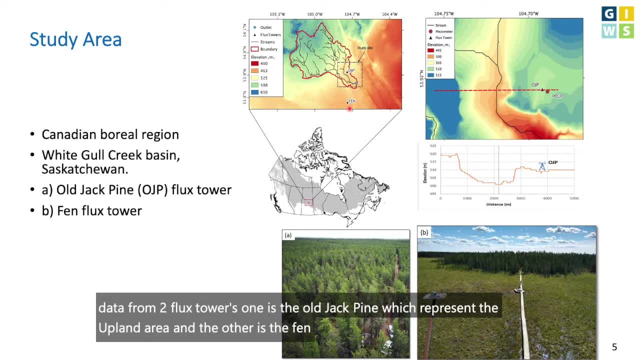 and the other is the fen, which represents the wetland component. Here you can see a focused view on the upland side and a real cross-section of the area there. For the modeling purposes we only considered one half of the cross-section and assumed the similarity between both sides. 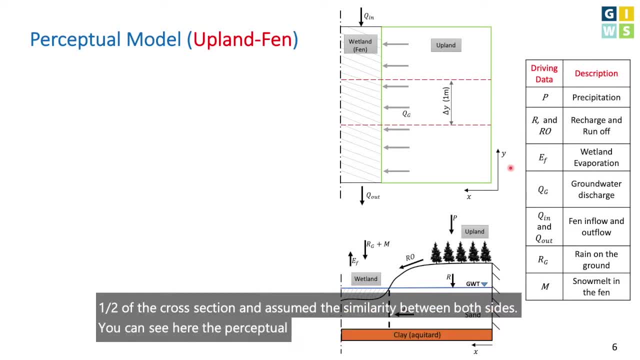 You can see here the perceptual model of the upland-fen system is shown using the two views: the top view and the cross-sectional view. The top view: here you can see the upland interacting with the wetland across this section through the movement of groundwater. 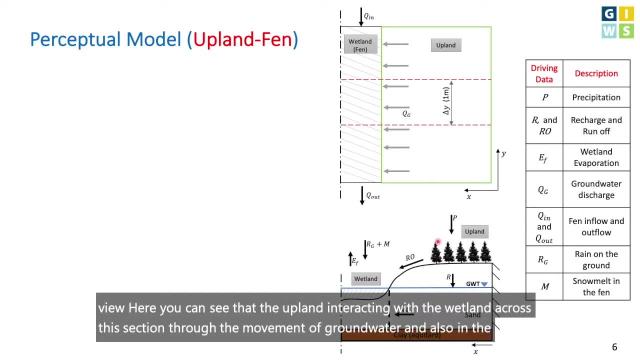 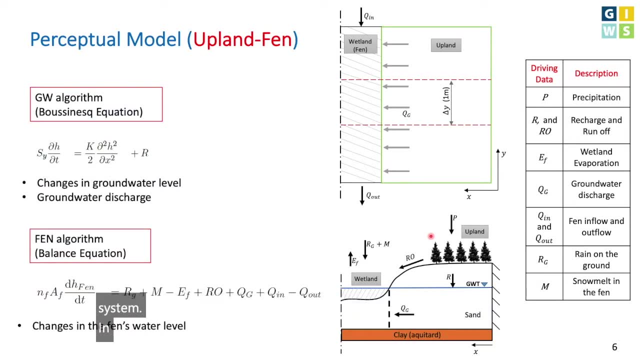 And also in the cross-section view you can see all the vertical fluxes that contribute to the system. In our model, we mainly have two options. In our model, we mainly have two options. In our model, we mainly have two options, two algorithms, one for the upland groundwater and the other for the fen water balance. 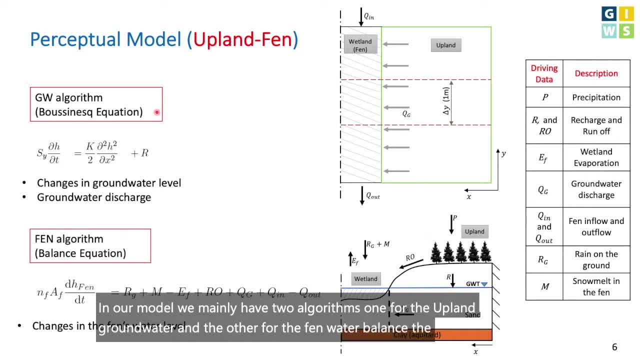 The groundwater algorithm is based on the Pozenitsky equation and is used to simulate the changes in the groundwater level and the groundwater discharge. The fen algorithm is based on the water balance equation and is used to simulate the changes in the fen water level. 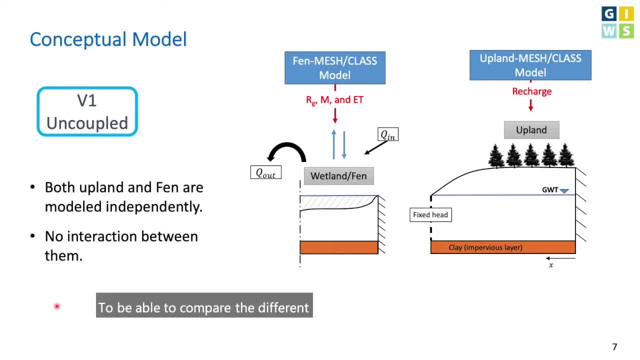 To be able to compare the different modeling approaches, we developed three conceptual models or three versions. Version 1 is for the uncoupled approach. In this model, the upland and the fen are simulated independently, with no interaction between them. For the uncoupled upland, the MeSH class model, which is the Canadian land surface model. 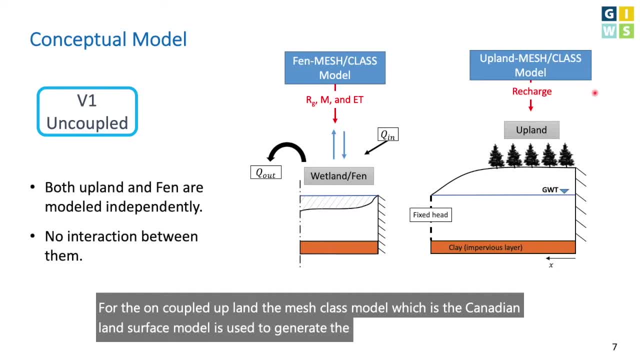 is used to generate the recharge values to drive the groundwater model. And here for the groundwater system we assumed an unconfined aquifer and assumed at the right boundary as a no-flow boundary and for the left side as a fixed head value. 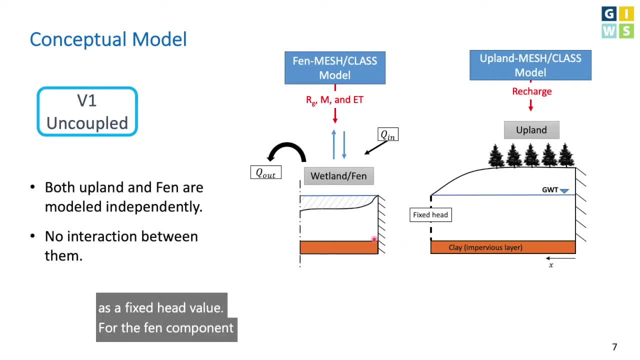 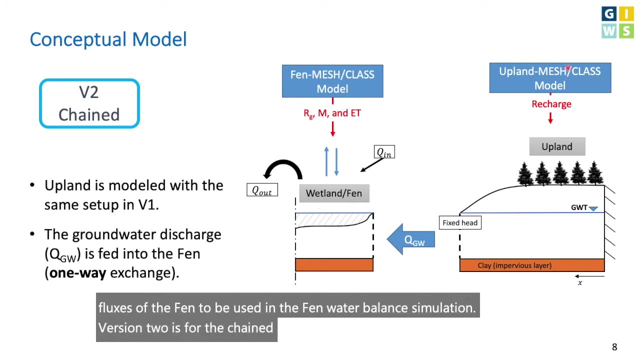 For the fen component. also the MeSH model was used to get the vertical fluxes of the fen to be used in the fen water balance simulation. Version 2 is for the chained model, And here the upland model is the same as version 1, and the simulated groundwater discharge. 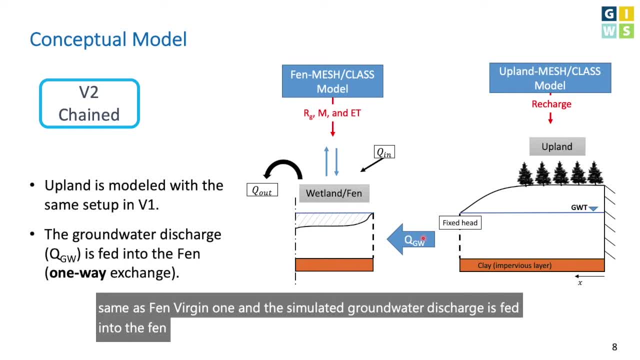 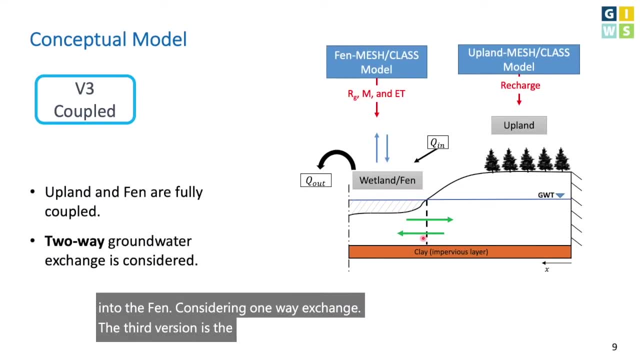 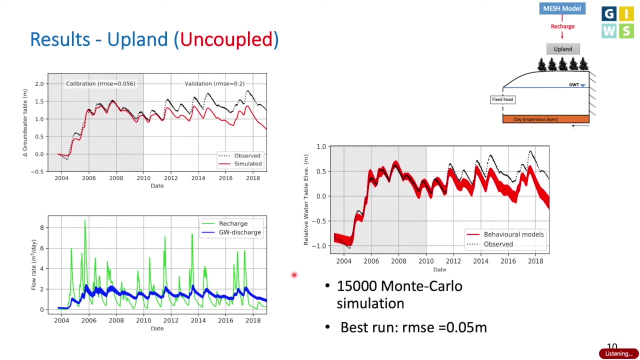 is fed into the fen, considering one way exchange. The third version is the fully coupled model. In this version, a two way groundwater exchange is considered. I'll start now by showing you the results. the uncoupled upland model. The model was calibrated and validated using 15,000. 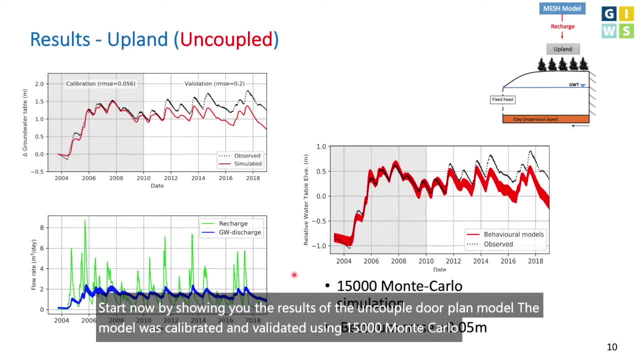 Monte Carlo simulations, The bistron had a root mean squared error of 0.056 for calibration and 0.2 for validation. You can see here for the validation period that after the year 2011, the model got exactly the same pattern of. 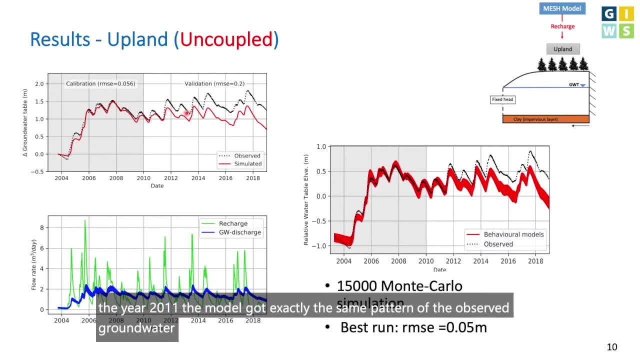 the observed groundwater table, with almost constant difference between simulated and observed, and we think that is because of some errors in the driving data at these two years that affected the rest of the simulation period. Out of the 15,000 runs, we found that 70 models can be considered as behavioral as they 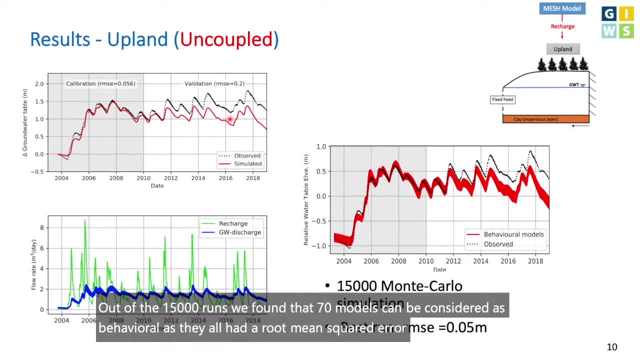 all had a root mean squared error below 0.1.. The behavioral runs were used to get the uncertainty bounds in the simulated groundwater discharge, here plotted in blue and compared here with the recharge values that drive the groundwater model. Also, they were used to get the uncertainty bounds in the 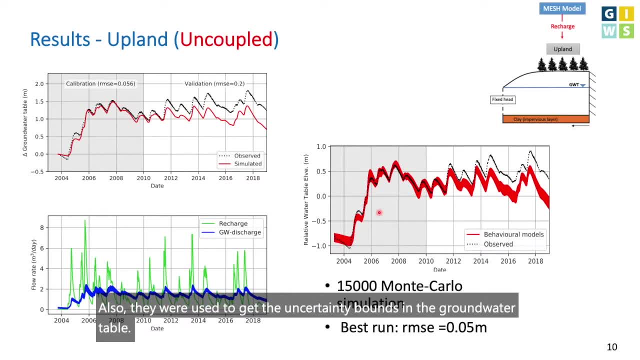 groundwater table. So actually using this model, we were able to get a little information about the upland component. Even we were able to have information about the co-ISf offsets of FO2 and their superspace balance needle fields possible. we were able to have information. 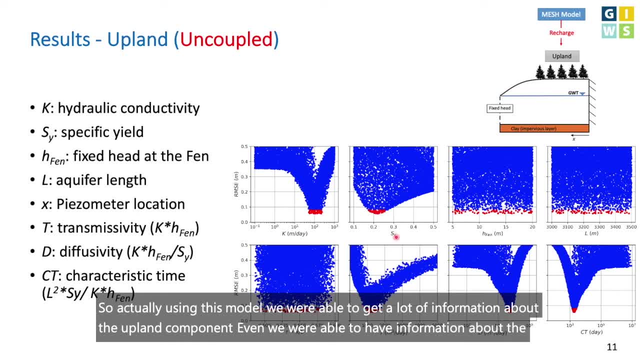 about the parameter's identifiability. So this plot here showed the identifiability of each parameter by plotting the parameter's values versus the root mean squared error for all the Monte Carlo simulations, And here the red dots represent the behavioral ones, The hydraulic conductivity and specific yield. 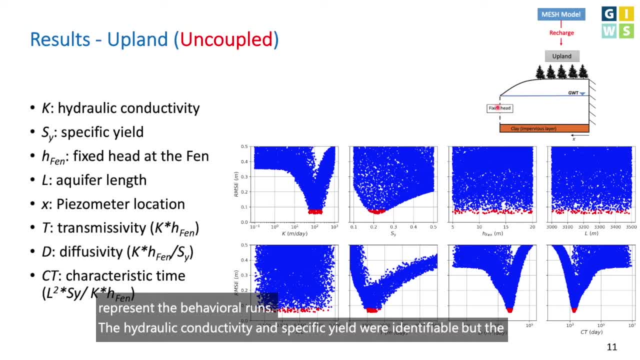 were identifiable, but the head value at the left side, the length of the aquifer and the exact location of the piezometer were not. We also tried to plot new parameters, which are a combination of identifiable and non-identifiable parameters. 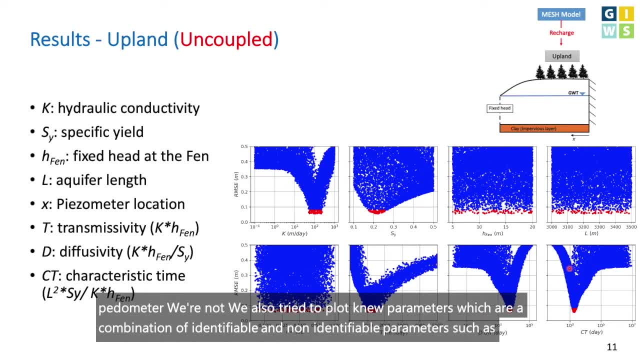 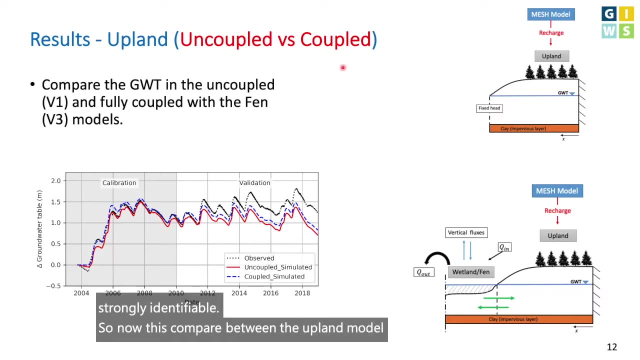 such as transmissivity, diffusivity and the characteristic time, And these three were strongly identifiable. So now let's compare between the upland model, the uncoupled and the coupled one. The same calibration parameters from the uncoupled model. 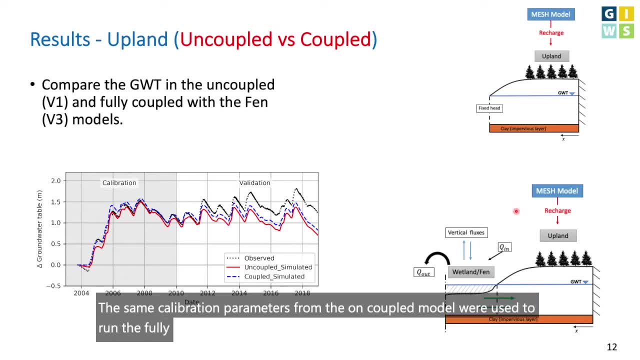 were used to run the fully coupled model And this is the simulated groundwater using both the coupled and uncoupled models. compared with the observations, You can see here that the coupled model has better match with the observations, but still there is no significant difference. 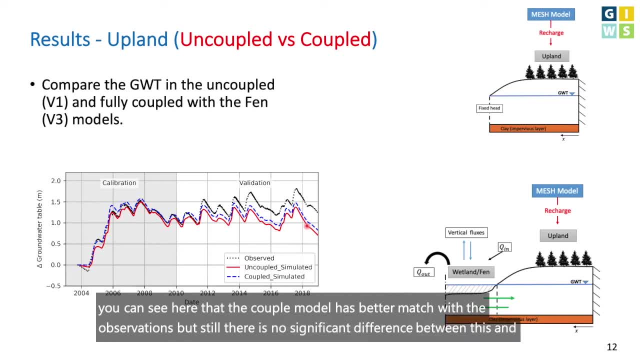 between this and the one simulated using the uncoupled model. So for the upland system, we can say that the uncoupled model is good enough and we're able to simulate the system and give out the information that we needed. It even allowed us to perform different analysis. 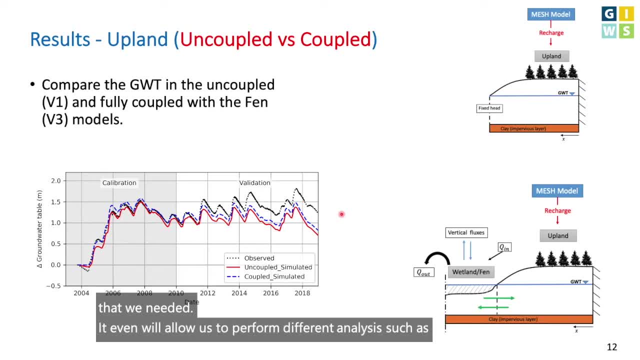 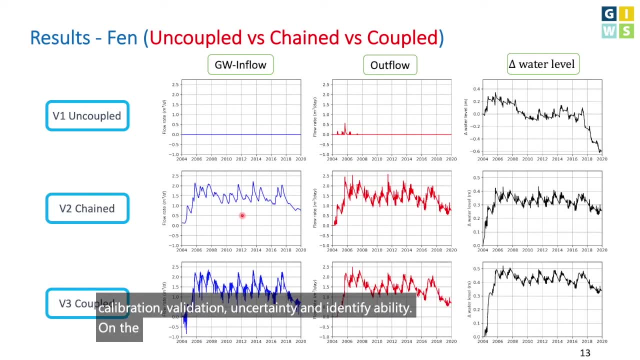 such as calibration, validation, uncertainty and identifiability. On the other hand, for the fan component, the uncoupled fan model, which has no groundwater inflow, wasn't able to get a reasonable result for the fan outflow and the change in the 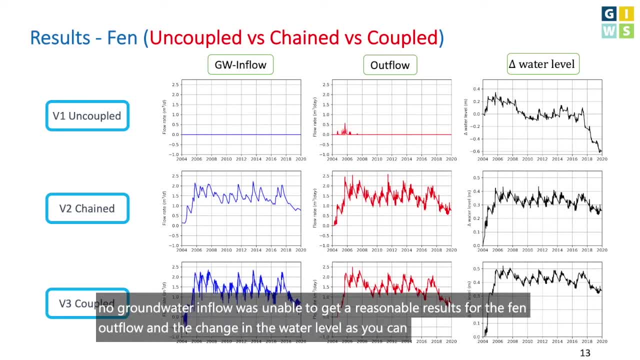 water level. As you can see, the outflow values were extremely low and the water level in the fan is declining, which is not representing the reality. But the chained and coupled models had a reasonably good simulation of the inflow, outflow and 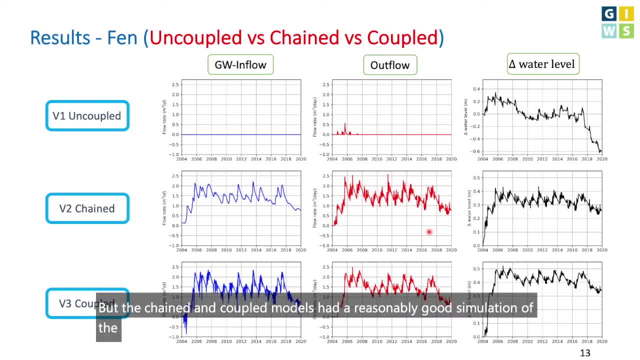 the water levels, with some differences between both. For example, looking here at the groundwater inflow, you can see that at year 2005, in the coupled model, the flow was reversed from the fan to the groundwater, which doesn't appear here in the 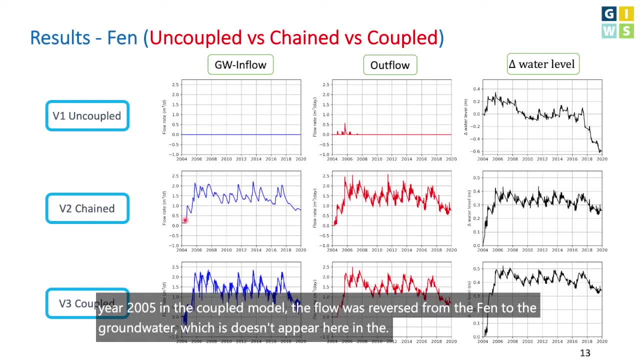 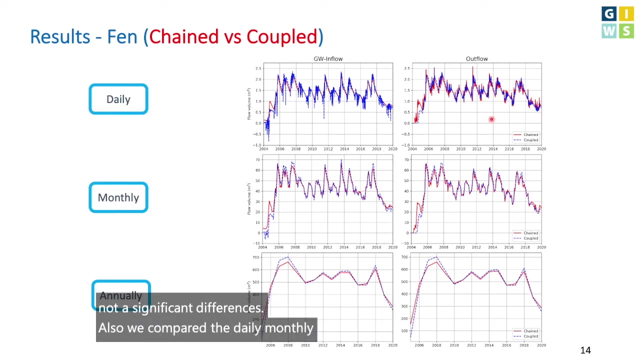 chained model, but that was only for one year of the whole simulation period. You can here also see the differences between the simulated outflow and the simulated water level in the fan. but after all all of these are not significant differences. Also, we compared the daily, monthly and annually ground inflow and outflow from the fan for 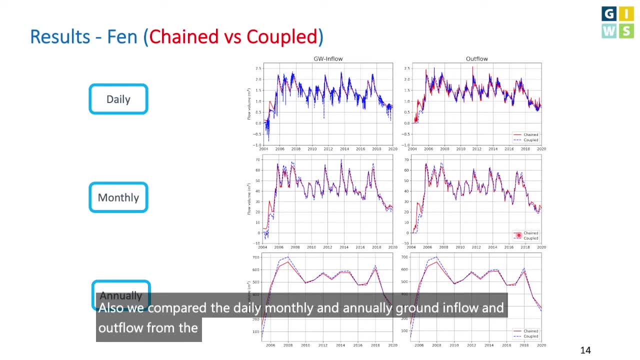 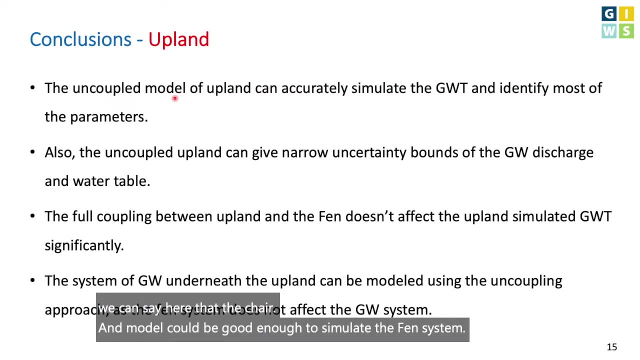 both models, The chained and coupled. But it's obvious that there is no significant difference between the two models. So we can say here that the chained model could be good enough to simulate the fan system. So finally, as a conclusion, we can say about the uncoupled model of the upland that it 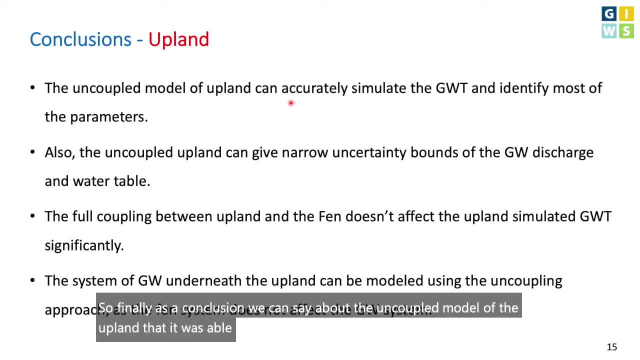 was able to accurately simulate the groundwater table and identify most of the parameter. It also was able to give an error uncertainty. The fan system is composed of a total of 10 points, so we can say that it is a pretty simple system. The minimum level of the fan is about 90% of the groundwater discharge and the groundwater. 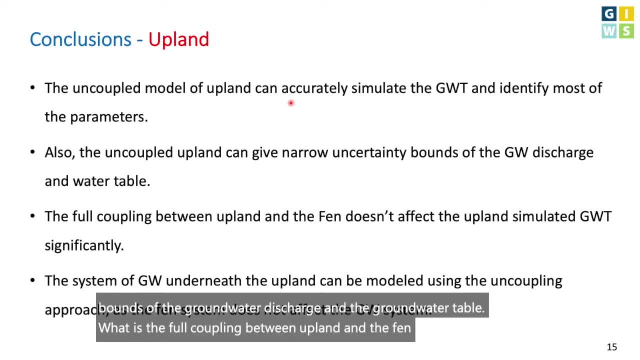 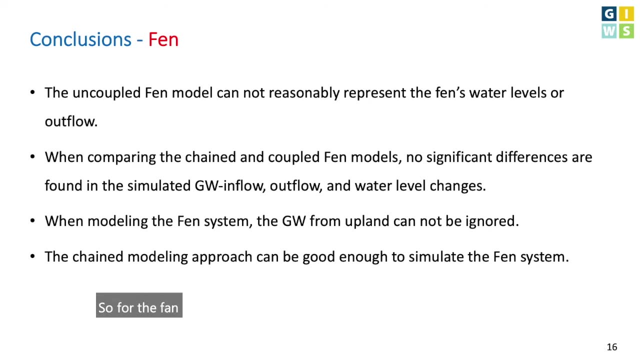 table. But the full coupling between the upland and the fan doesn't affect the upland significantly. So we can say that the groundwater underneath the upland can be modeled using the uncoupled approach. So for the fan system we found that the uncoupled fan model can reasonably represent 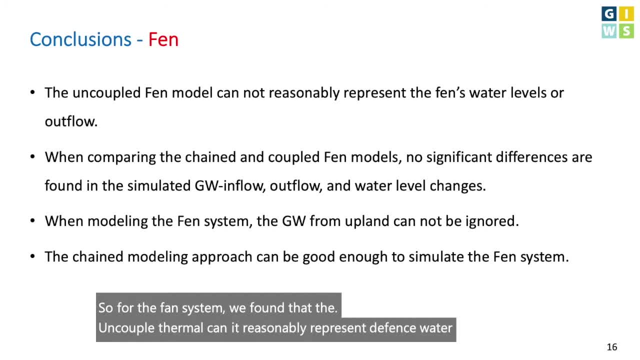 the fan's water level or the outflow. So we also found that the uncoupled model cannot reasonably represent the fan's water level or the outflow. But when comparing the chained and coupled models, both models were able to get a good.